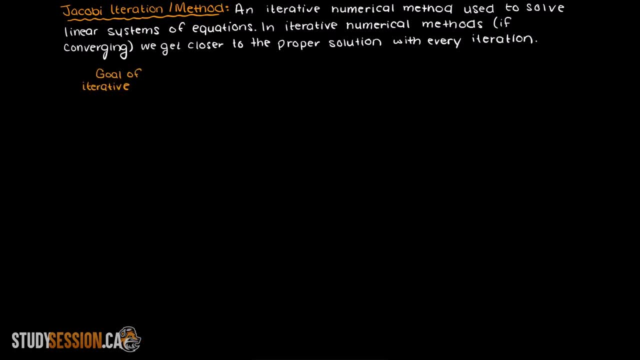 to get from our starting position to our final answer, and every step that we do take will be one towards minimizing the error of our problem. Then we will continue this iteration until we reach an acceptable level of error. Before I begin, I should note that you cannot. 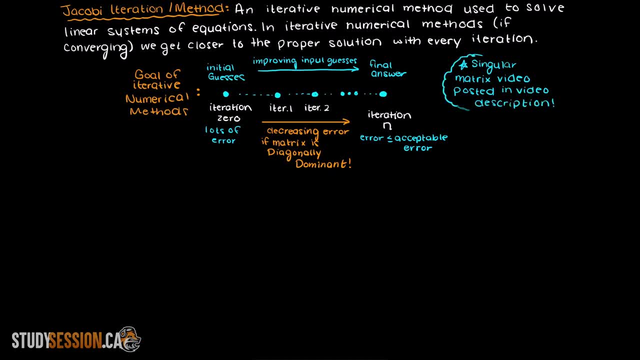 use Jacobi Iteration when you have a singular matrix. This means that the matrix has no solution, and I will post a video in the description below if you want to learn more about singular matrixes. So the steps to solving a linear system. 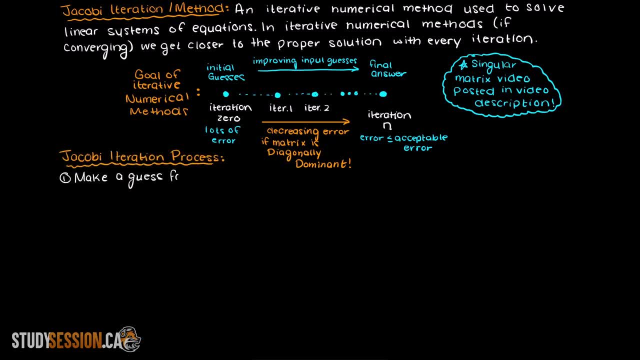 of equations using Jacobi Iteration are the following: Firstly, we make a guess for every value in your x matrix. Therefore, we need to assume a value for x1,, x2, x3, etc. for as many x values as you have. Let's call our initial. 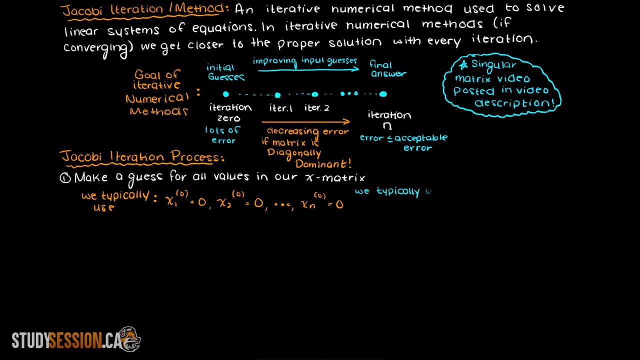 iteration 0, as many programming languages like Python have zero indexing, meaning we start counting from 0 in them. However, if you are using MATLAB, begin at 1, as it does not have zero indexing. A typical starting guess is just a zero matrix, unless we have some additional information. 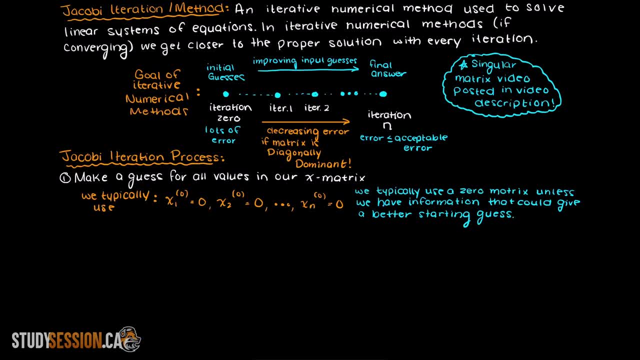 about the problem that could help our guess. The benefits of having a better starting guess is that we can achieve our final solution in less iterations. Now step 2, we need to write all of our independent equations and have them all solved for different. 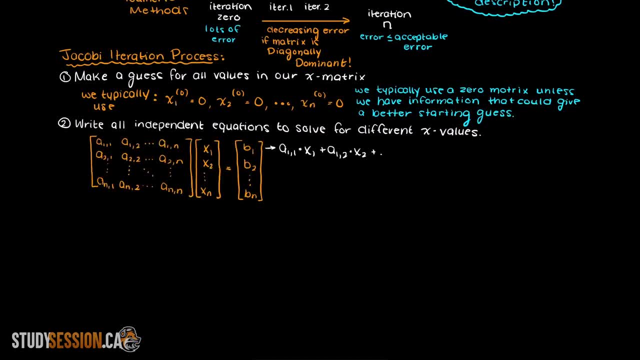 x terms. So you can see here that I have done that Step 3, so once we have rewritten our system of equations, it is often wise at this point to create a table to summarize all of your relevant information. This is how I would. 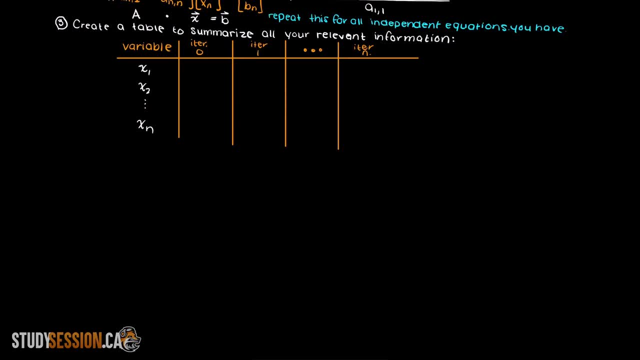 recommend making your table. however, as long as your table has all the important information on it and you understand it, that is all that matters. Step 4, we are now ready to solve for our iteration 0. We plug in our assumed values into our system of linear equations and these output values are going to be the values used. 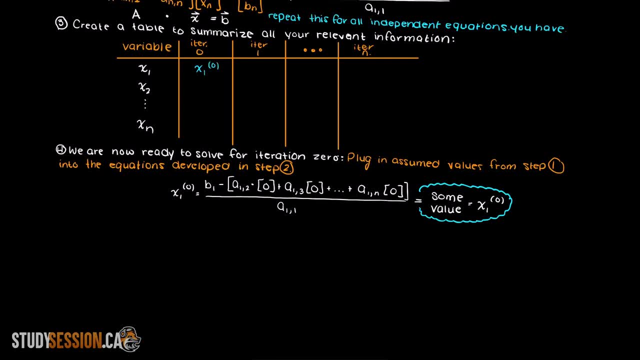 in our next step or our next iteration, Step 5,. as I said, these new found x values will be our new guesses, So we will repeat what we completed before and plug these values into our main equations again. I should also note that sometimes you will see the iteration number denoted in parentheses.